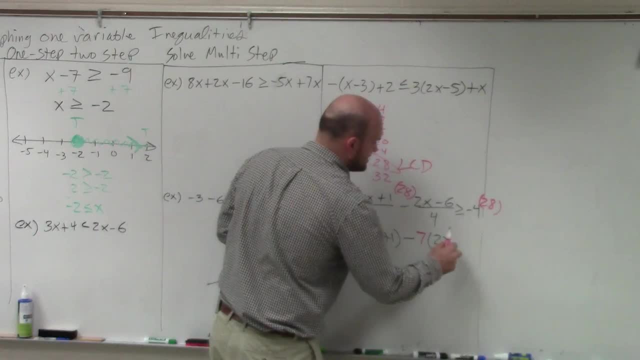 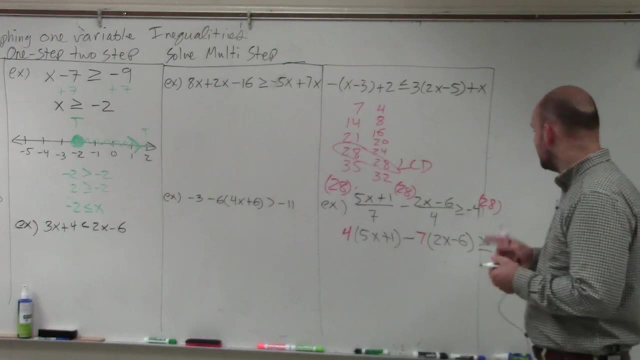 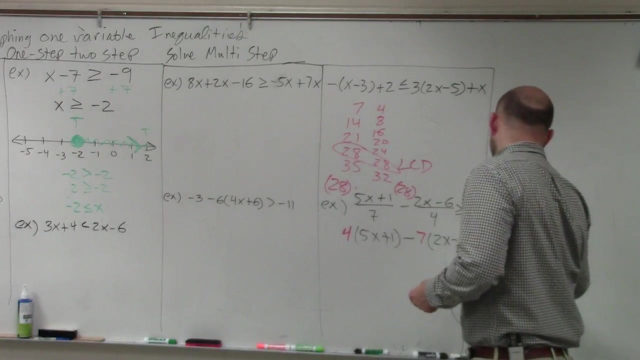 7. And then that's going to still be multiplied by 2x minus 6. And then that's going to be greater than or equal to negative. 4 times 28 is 28.. That's going to be 56.. That's going to be 112.. And that's. 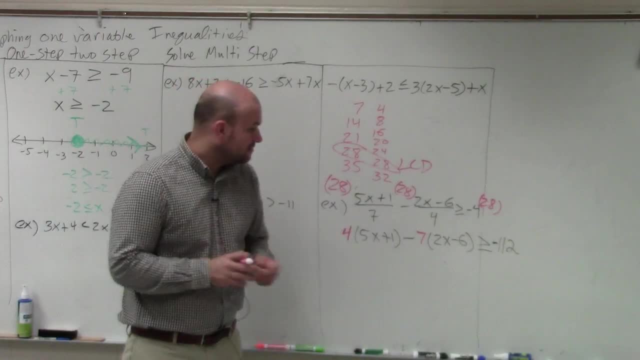 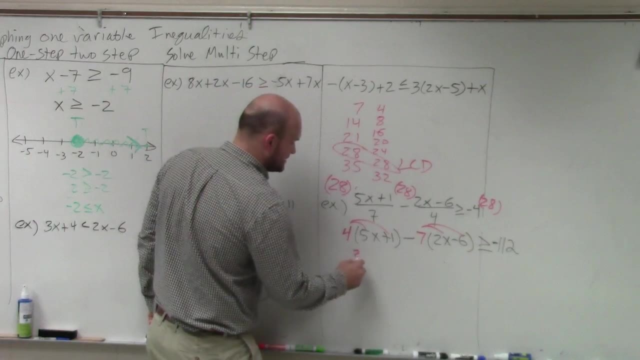 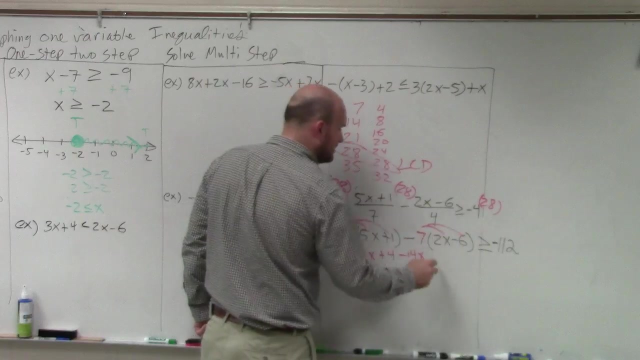 a negative. Now we apply distributive property: Multiply, multiply, multiply, multiply. So therefore we get 20x Plus 4. Make sure this is a negative 7.. So that's a negative. 14x, That's going to be plus. 42 is greater. 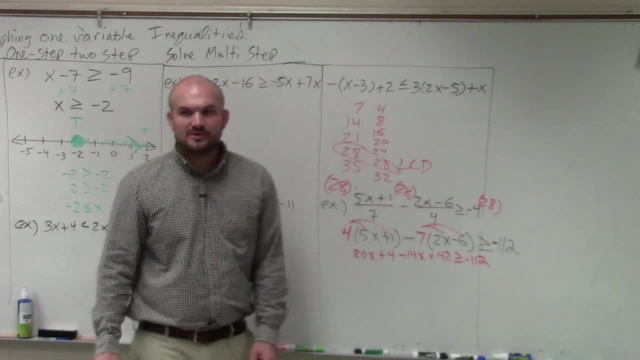 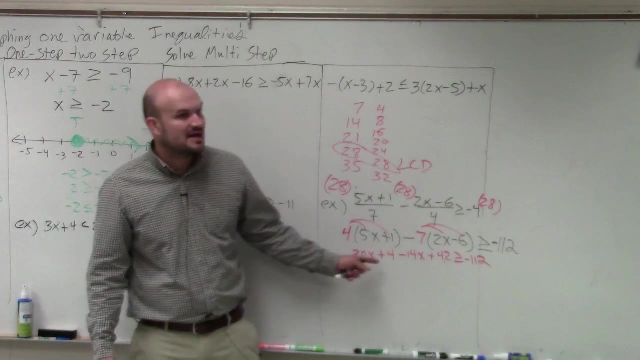 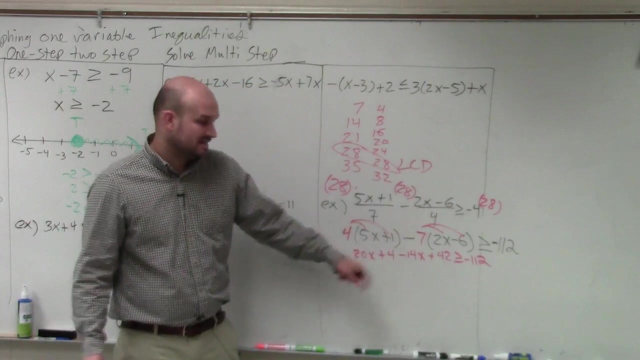 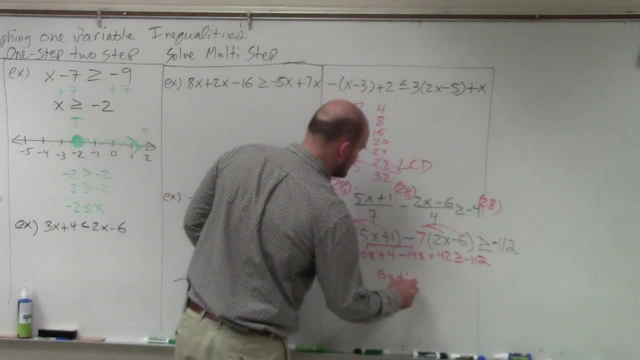 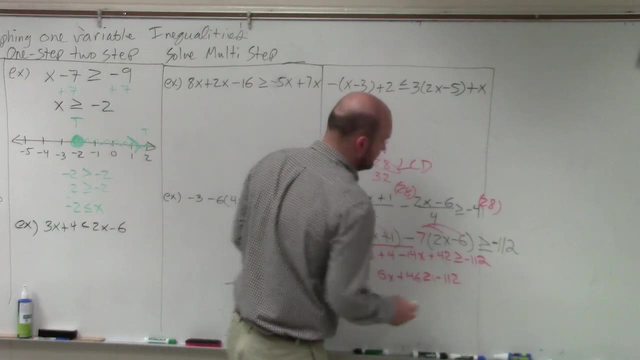 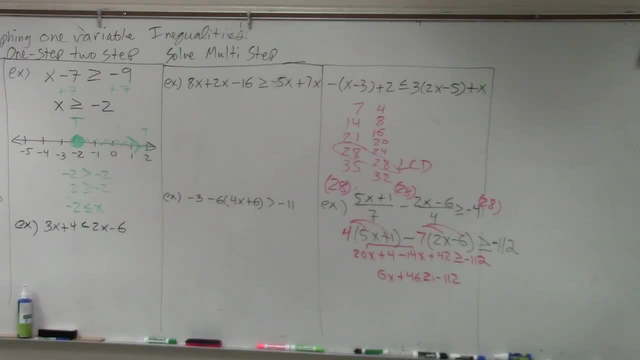 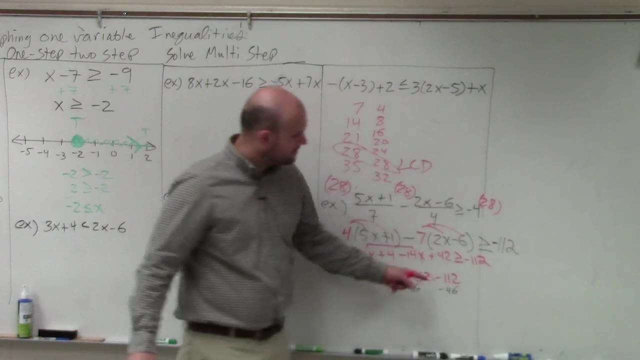 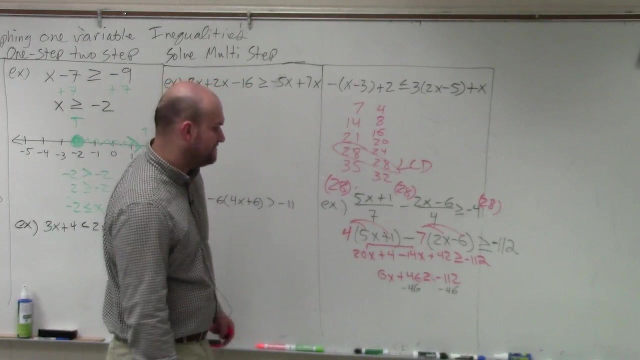 It's a little bit bigger numbers, but hopefully you should be able to do this. So therefore I'm going to minus 46.. Basically, when you have a negative number minusing another number, it's like adding it. So that's going to be 158.. 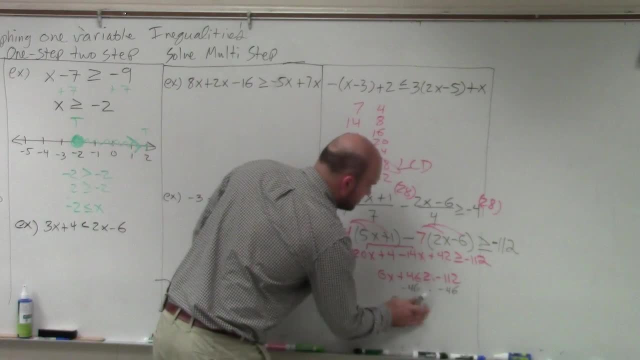 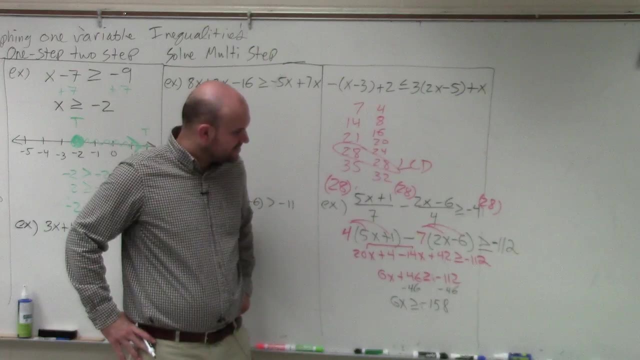 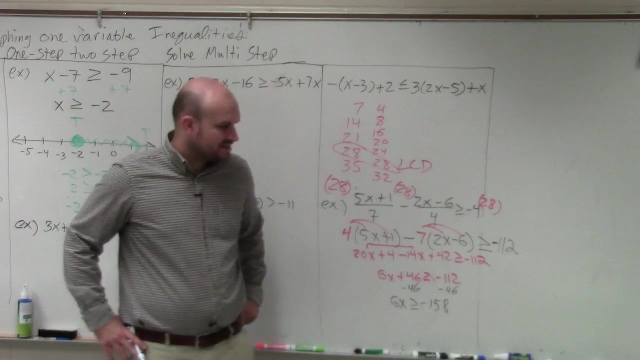 6x is greater than or equal to 1 negative. Let's do 60,, 120,, 180.. How many times does it go into it? Say it goes in. No, it doesn't go into that, does it? 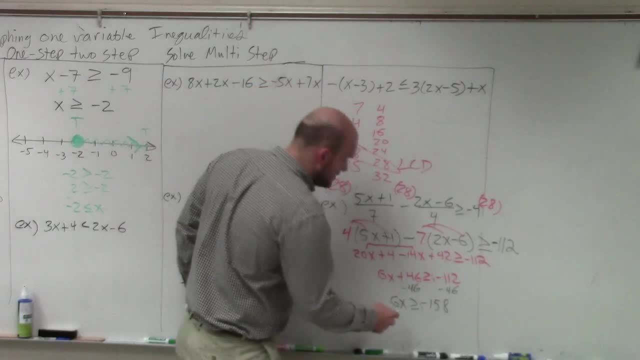 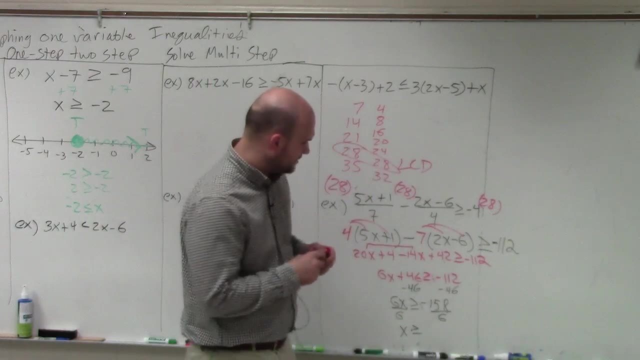 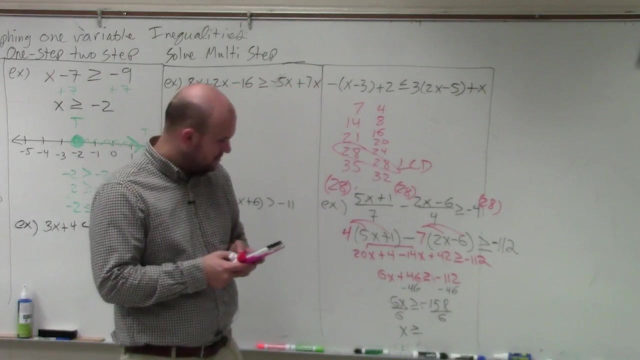 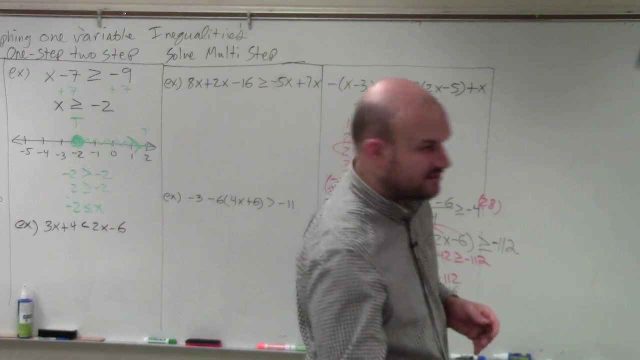 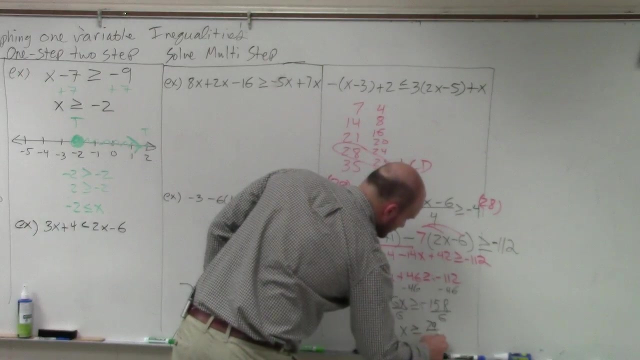 Not evenly. Huh, Not evenly. no, No, not evenly. OK, Yes, Let me just take a look at this. I'm getting 79 over 3 as the reduced fraction, which is approximately 26.33.. 26?. 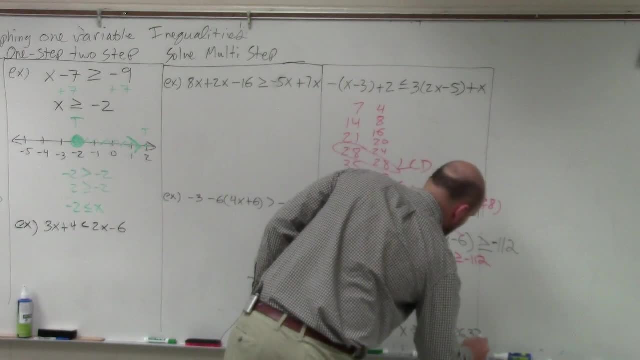 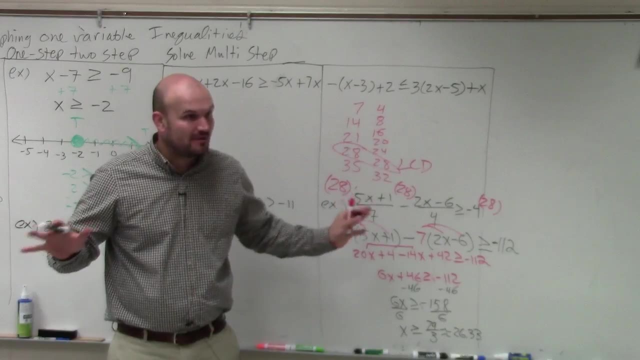 26.33.. 26.33.. So one thing I want you guys to understand about when you have a decimal, that is OK. It is OK to have a decimal and graph it. There's nothing wrong with that. Look at your number line. 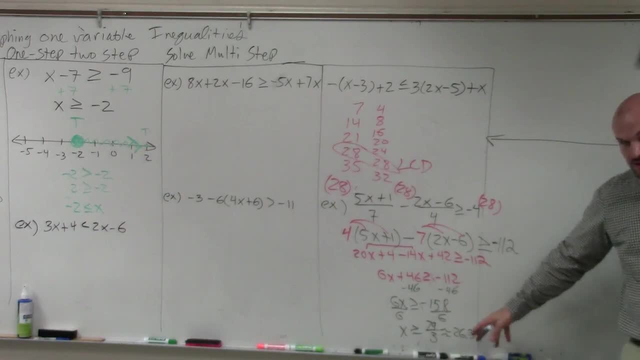 Now, if 79.3 is the fraction, here's your decimal. Can we put the number on 26?? Can we put the circle on 26?? No, it's 0.33.. Can we put on 27?? No. 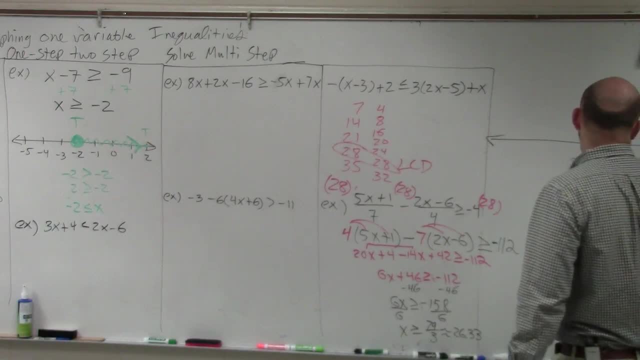 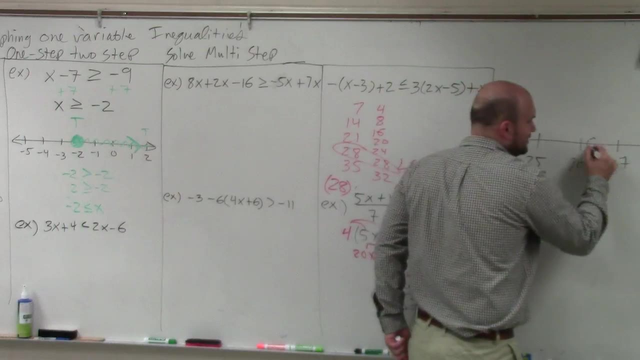 So what we'll do is we'll say: here's 26., Here's 26., Here's 27.. Here's 28.. Here's 25.. 26.33 is in between 26 and 27.. Right, It's in between them.